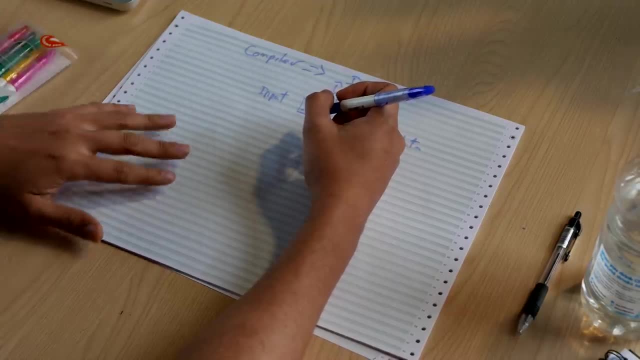 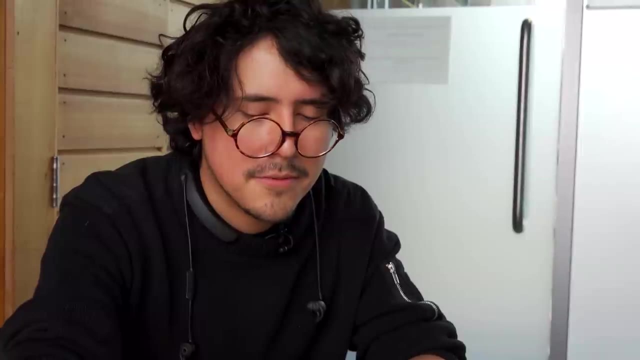 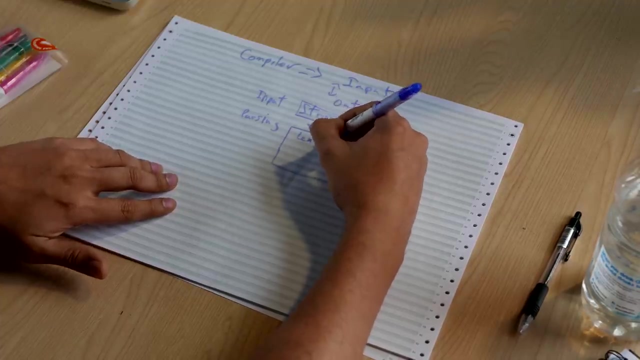 The first part in the compiler. the basic stuff that a compiler should do is essentially parse the input, And here the string, let's say, for example, needs to be able to be analyzed, And this has several steps In order to handle the string in the best way for the system. you have lexical analysis. 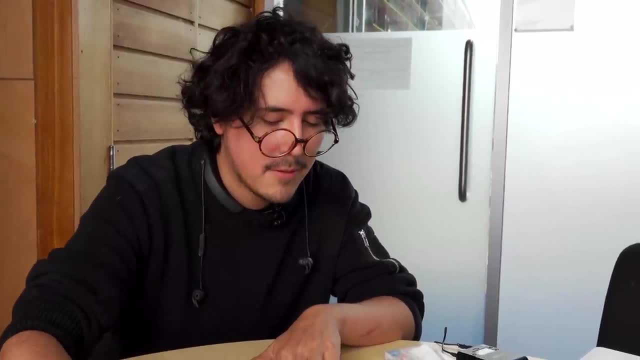 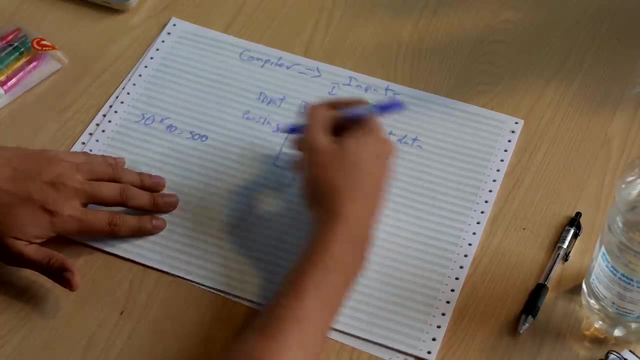 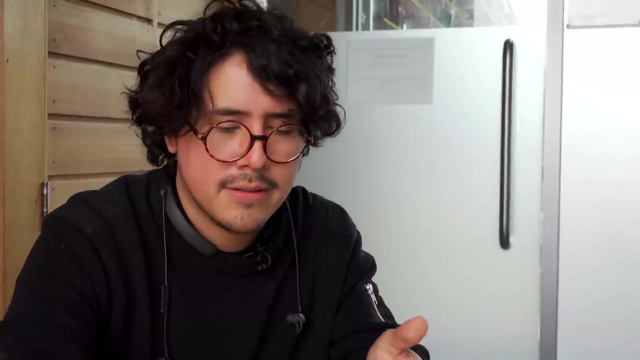 of the string. So say, you have a given multiplication, 50 times 10 equals 500. And this is a string. First, what it's going to have to do is lexical analysis, And here there's a particular reference to how humans can actually 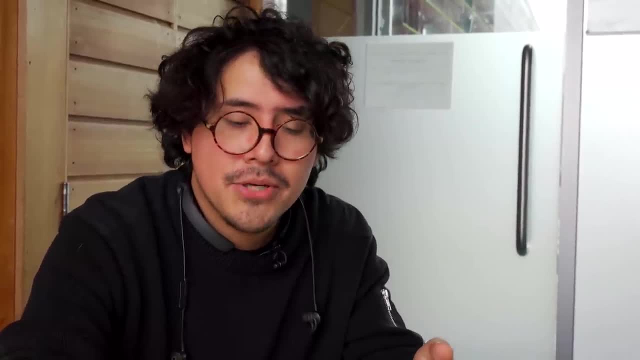 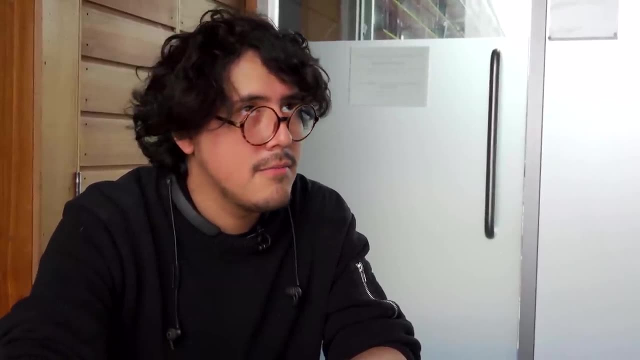 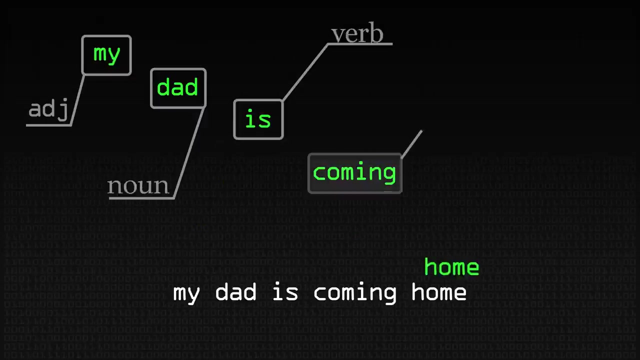 um understand information. A computational interpretation of how we understand it would be to like analyze each term. So like you have the sentence my dad is coming home And you classify those into verbs, adverts, nouns, etc. What the parser does essentially is do lexical analysis, which essentially means creating 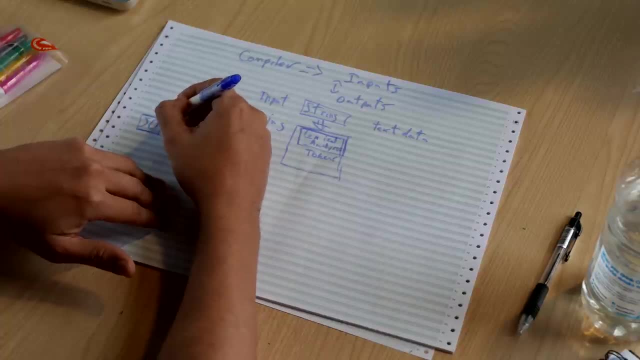 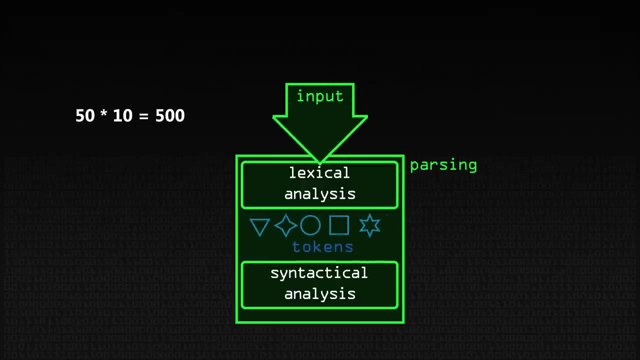 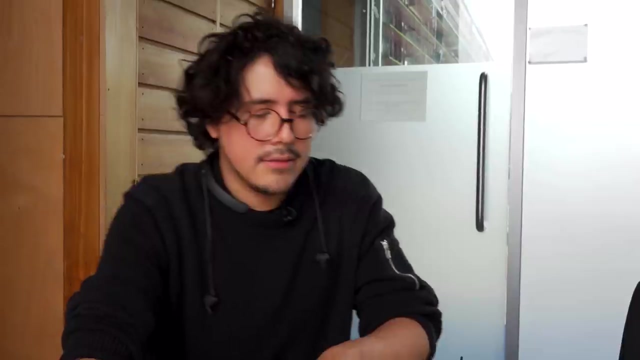 tokens. Tokens are each of the elements on the string. So, like 50, the multiplication sign 10 equals 500. And it needs to be able to do this because, at the end of the day, the string goes through a syntactical analysis. 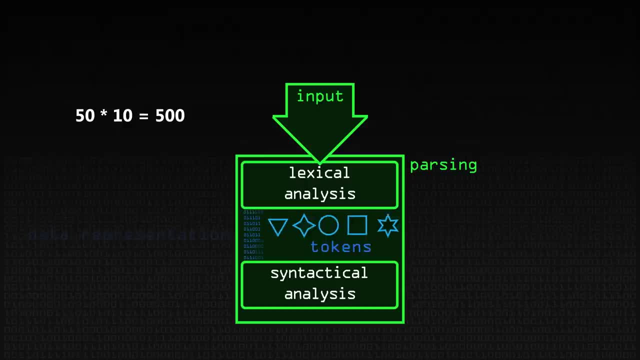 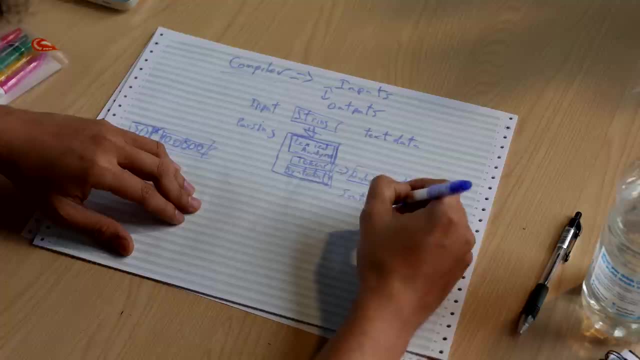 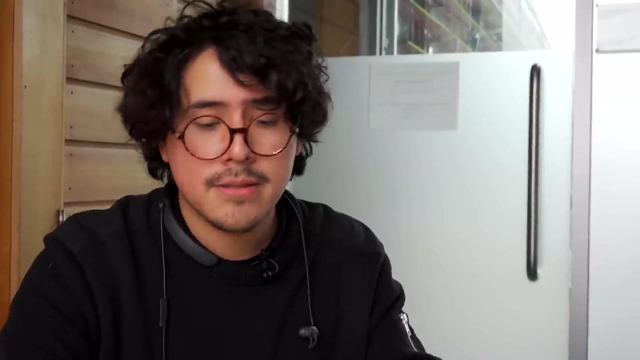 The tokens create some sort of data representation, And this data representation, in order to be able to be translated, it needs to be put through syntactical analysis. This is the part that's really interesting, because syntactical analysis means in humans as well as in computers. 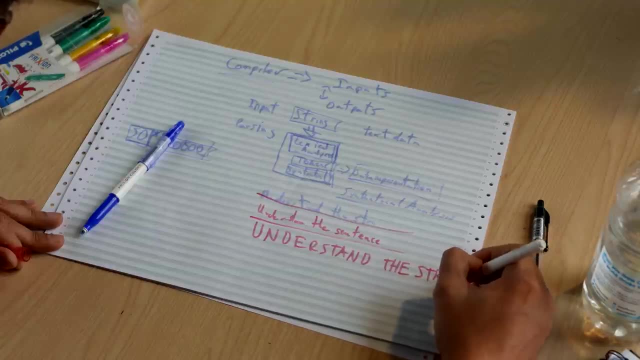 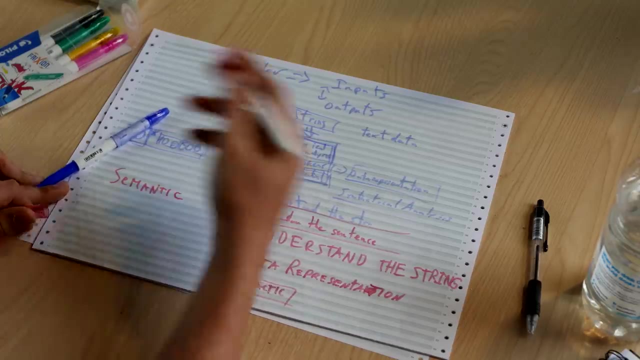 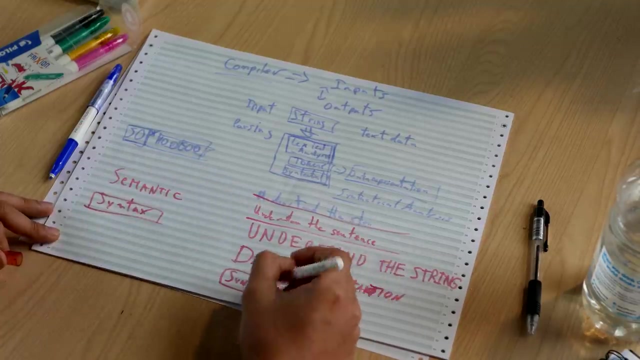 That you understand the string, understand the sentence. let's put it that way. Why is this important? Because semantics, meaning the actual outcome, what it means to understand a sentence, comes out of syntax, And syntactical analysis is basically done through a reference to context-free or any. 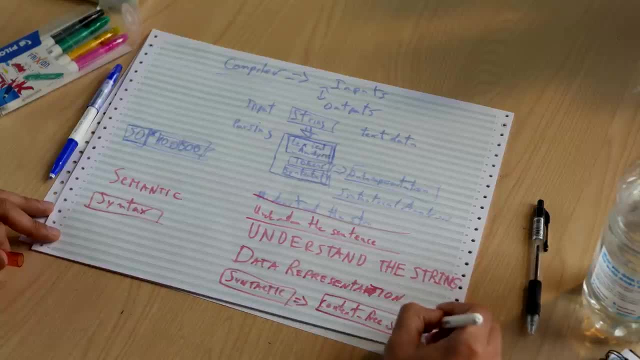 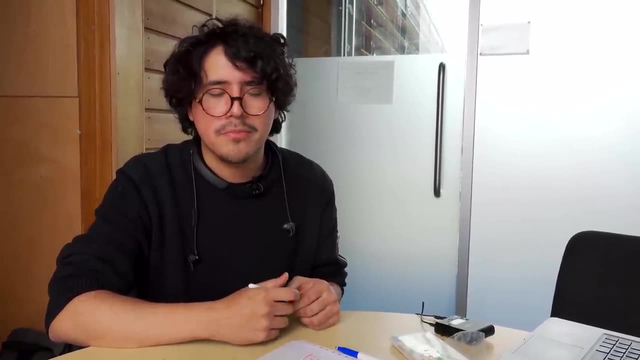 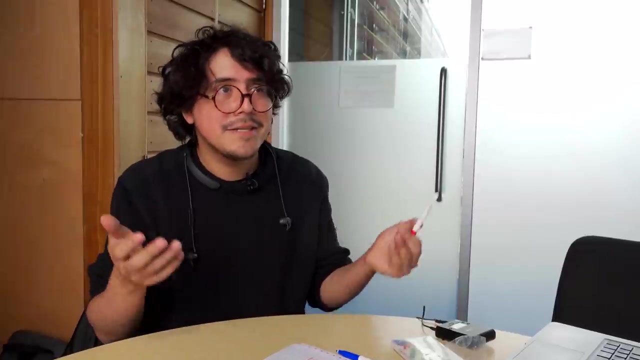 kind of grammar, really Context-free grammars, usually meaning that if someone speaks to you in French and you don't understand French or don't have that module in your head, you won't be able to parse it, So that data representation will have some sort of representation, will be like a sentence. 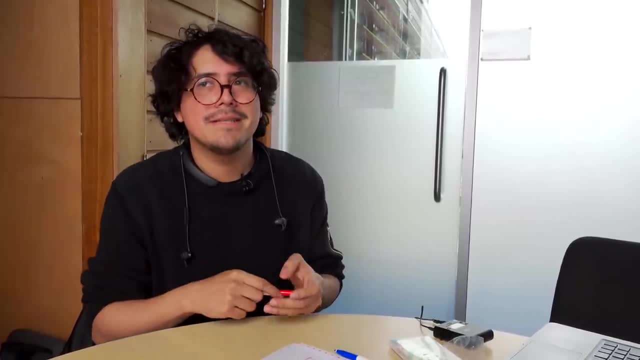 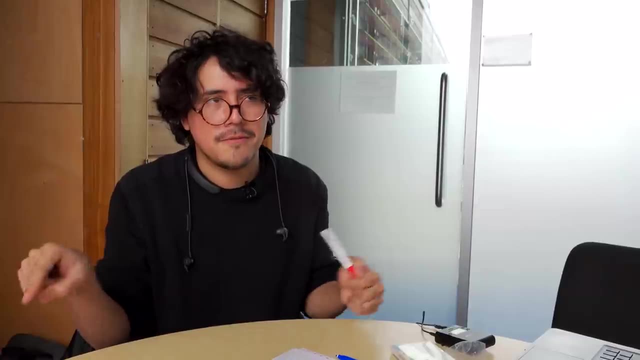 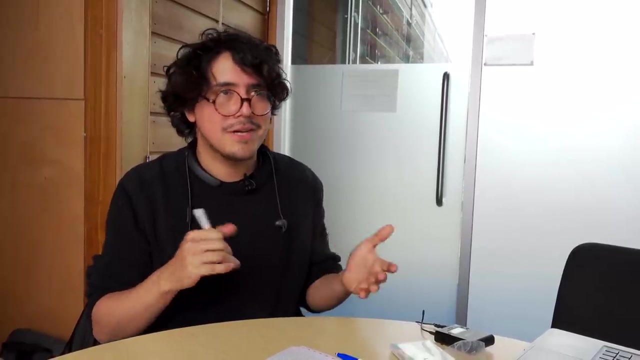 You can understand it through being a sentence, but you won't be able to extract any kind of semantic content from the syntax of strings. You can say they are letters, You can say they are words, You can say it's a sentence. You can say: 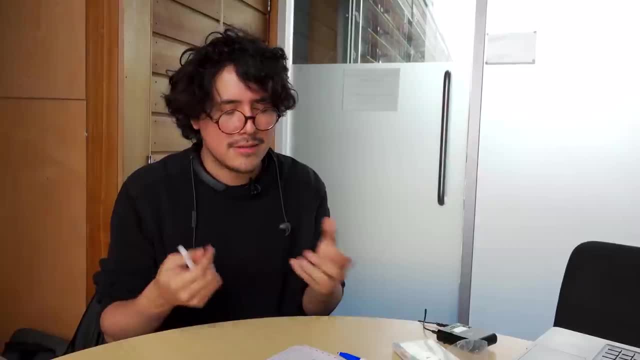 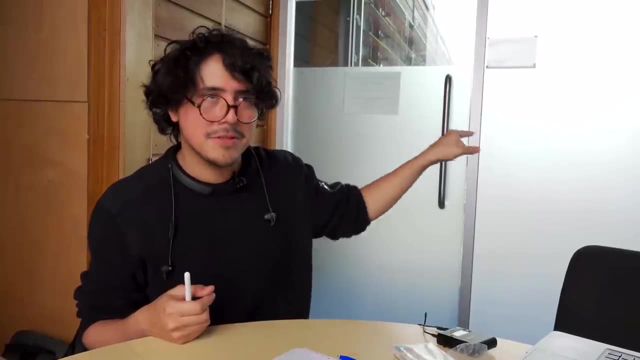 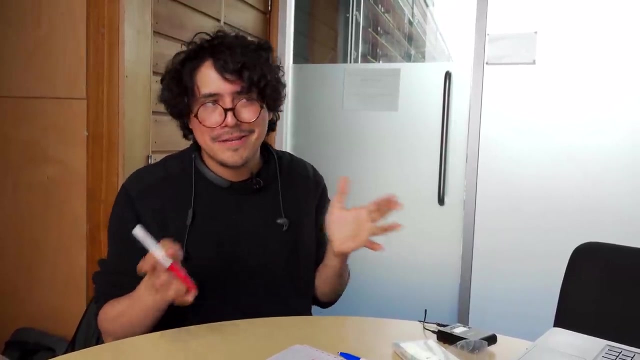 You must have some content. Obviously, with humans there's some ambiguity, as they have. like they can say: this is a door, This is a door, And you have the human pointing towards a door. So, but it's saying in French, hence you can do some abductive inference there and like: 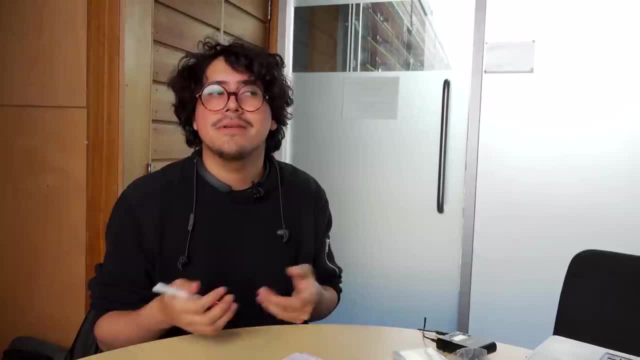 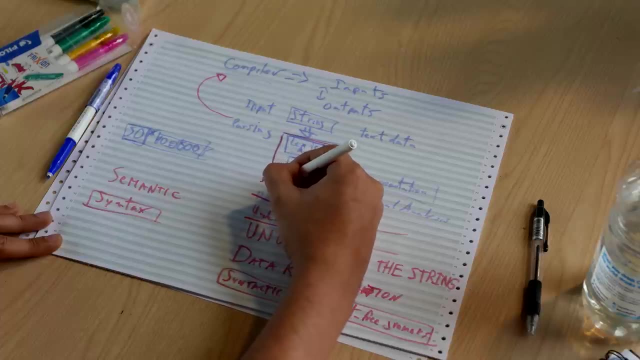 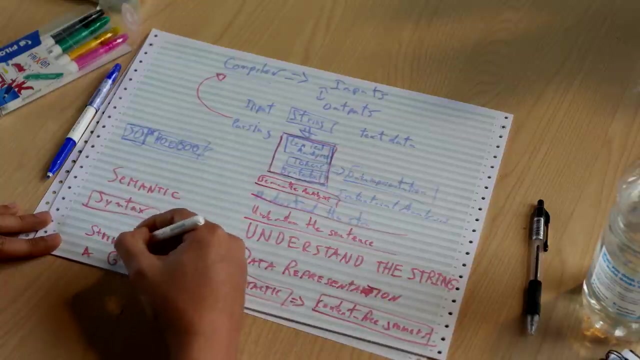 make sense. However, it doesn't. it doesn't mean that you're understanding the semantic content, And this is all a part of compilers. At the end of the day, The compiler does a semantic analysis after it's checked that the string conforms to the. 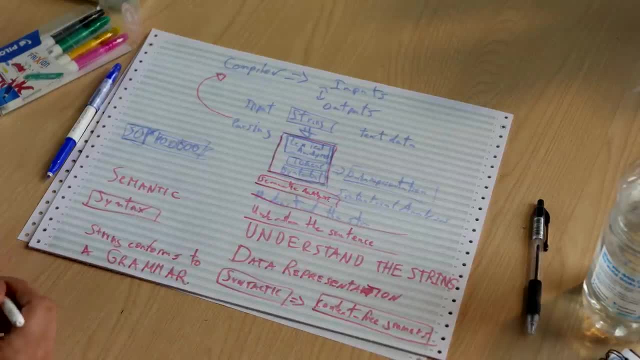 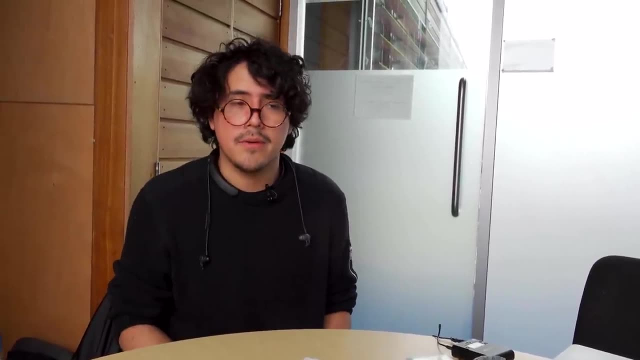 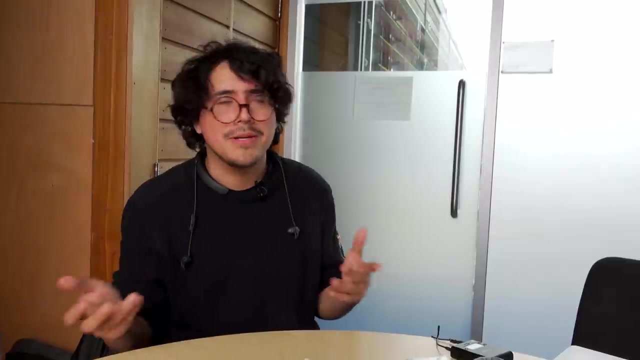 grammar inside of the system. And that's what parsing is The thing about: compilers and parsers etc. and the difference between, I guess, humans is that, while we can certainly take a computational angle and interpret our humans as essentially computers And 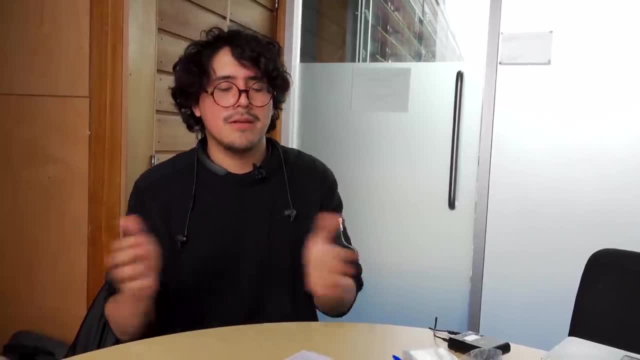 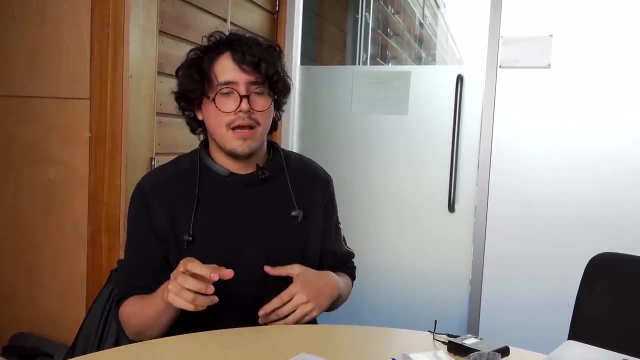 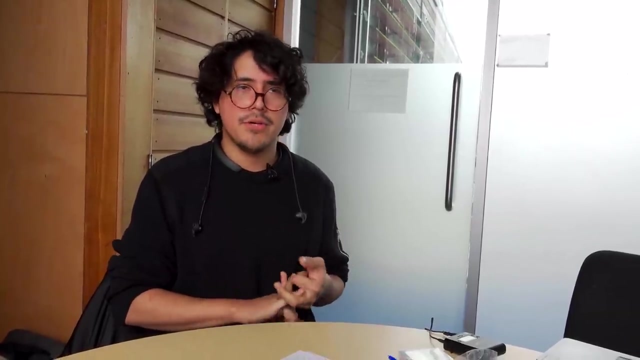 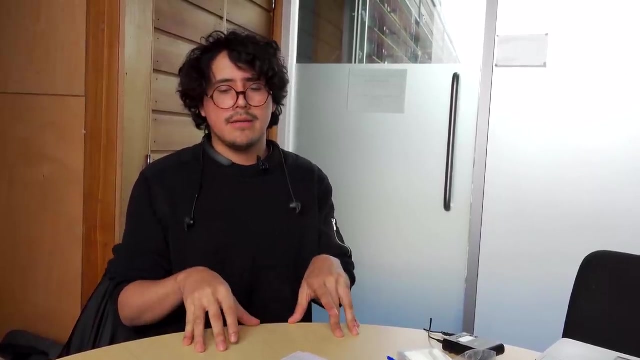 There are some similarities between how humans understand these things and how computers do. There is a crucial sense in which humans can tolerate ambiguity, can tolerate pragmatics, can tolerate different kinds of situations where informational content can be inferred, But in the case of computers, ambiguity becomes a matter of insecurity. 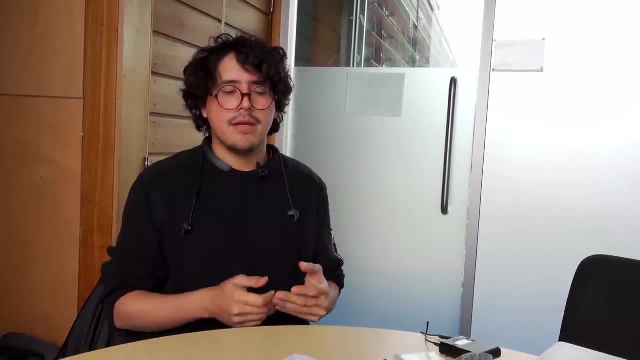 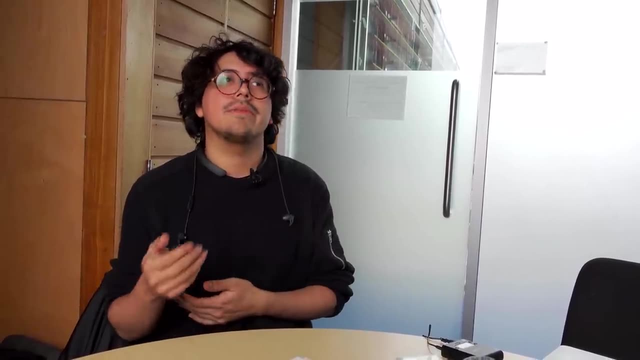 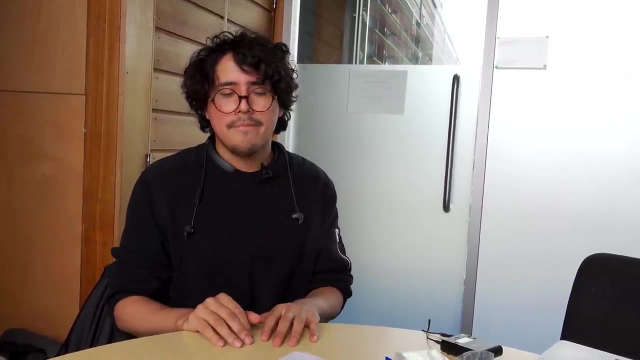 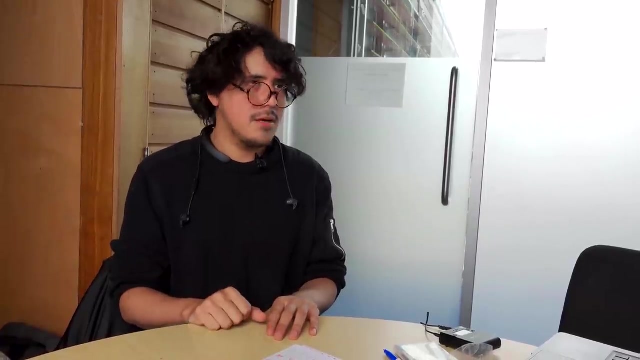 And There is an insecurity in not properly parsing inputs because someone, someone, didn't design a specific parser to understand a given string based on a grammar. that creates a lot of vectors of attack for- let's call them black hat actors, because there are, there are many ways in.